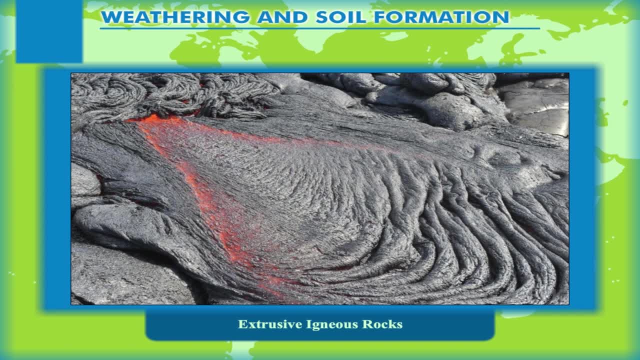 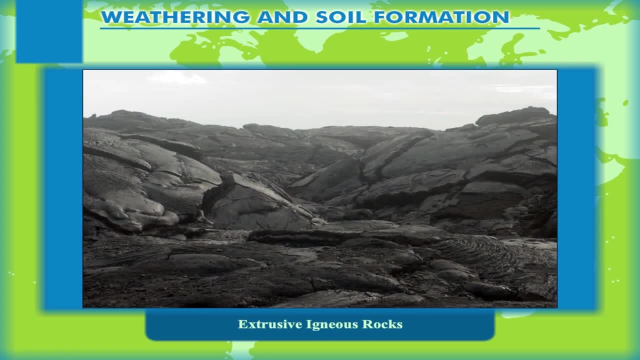 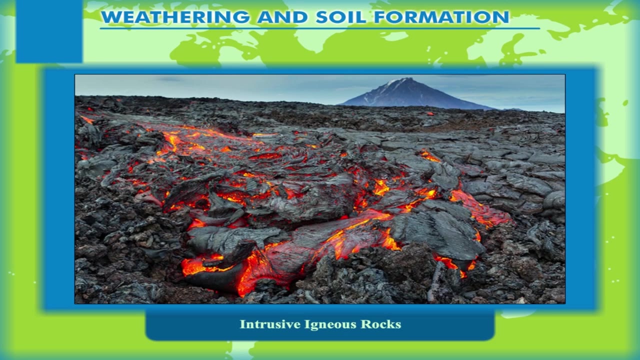 During the volcanic eruptions. when magma erupts and on reaching the earth's surface, it cools and solidifies. As a result, rocks are formed on the surface, known as volcanic rocks, Intrusive Igneous Rocks. They are formed by the solidification of magma. 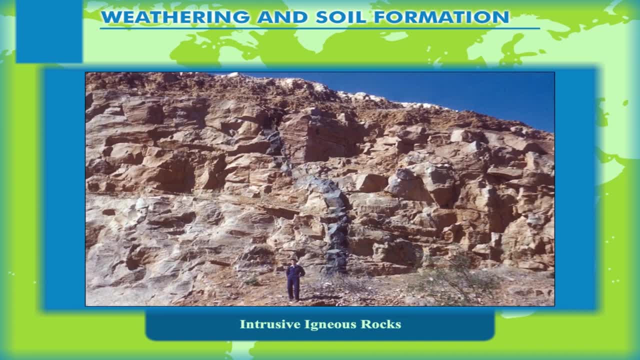 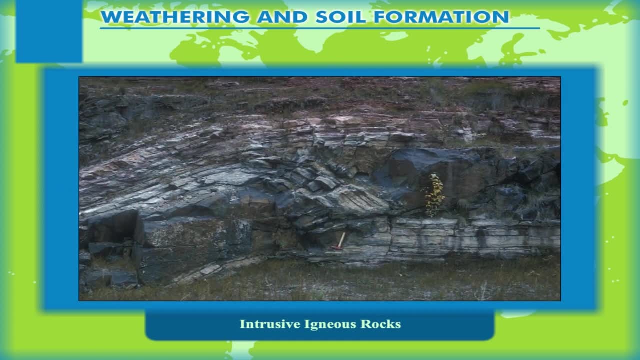 They are formed by the solidification of magma. They are formed by the solidification of magma below the surface of the earth, in the cracks or joints Inside the earth. magma cools very slowly and, as a result, forms crystals of large size. 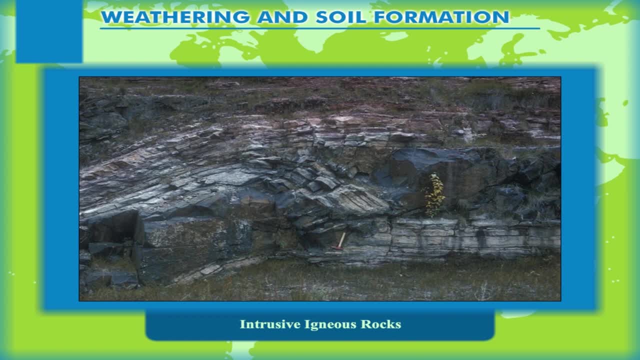 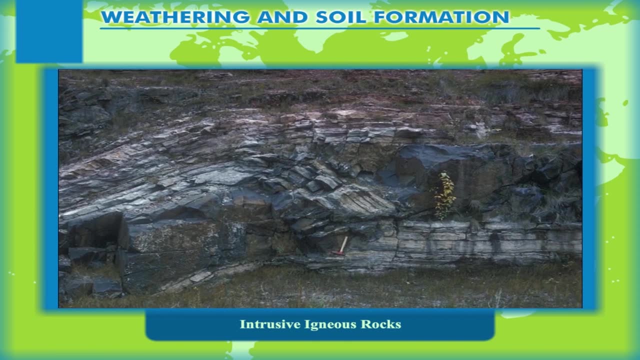 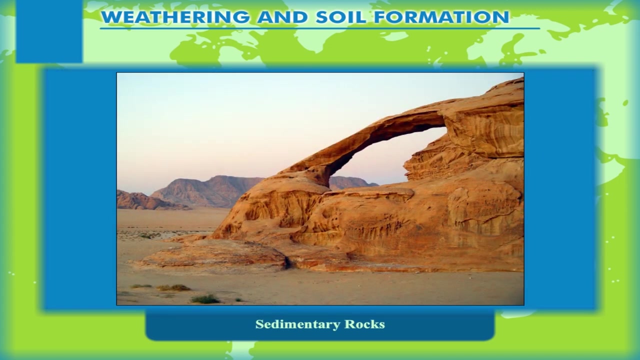 Sometimes the magma solidifies at a great depth. Due to very slow cooling, large size of rock crystals are formed very deep down. The deep-seated igneous rocks are called plutonic rocks, Sedimentary rocks. They are also known as secondary rocks. 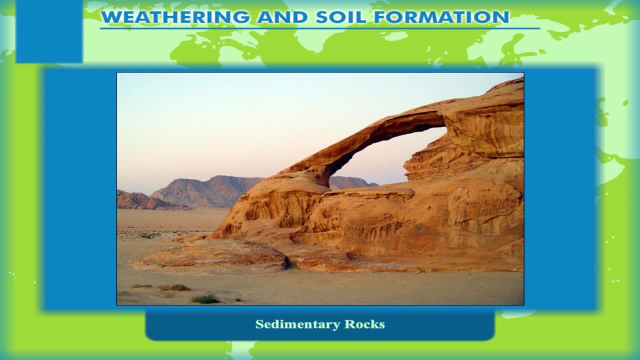 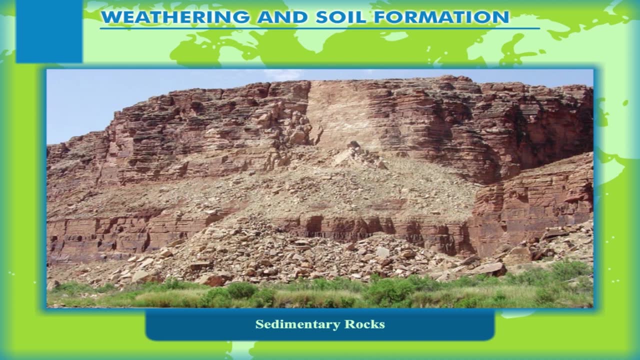 because they are formed from the sediments derived from the pre-existing rocks. Igneous rocks are exposed to the forces of nature. These forces break the rock on the surface of earth into small pieces. These small pieces turn to tiny particles with time. 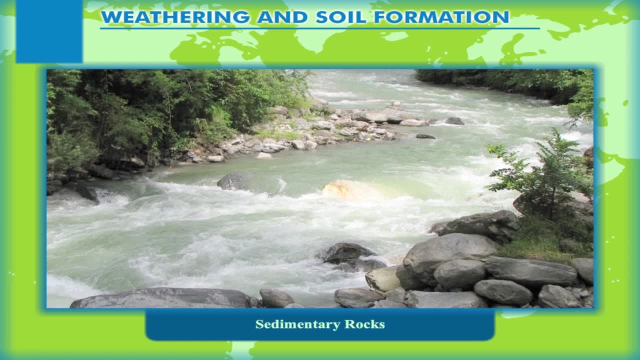 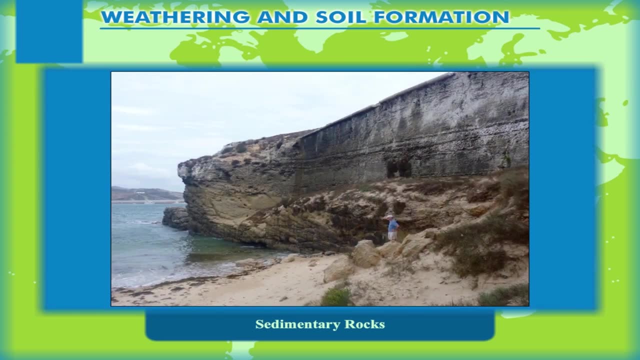 These tiny particles are transported by agents of nature like rivers or winds, and are deposited at certain places. The deposition of such materials occurs in layers. That is why they are called stratified or sedimentary rocks. These rocks often contain fossils of animal and plant life. 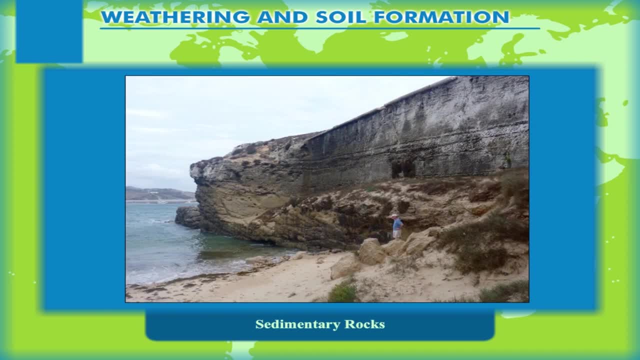 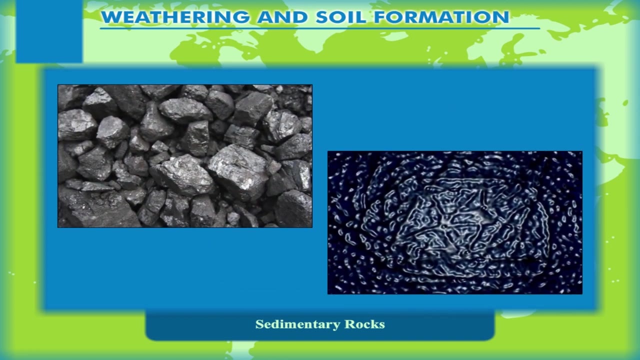 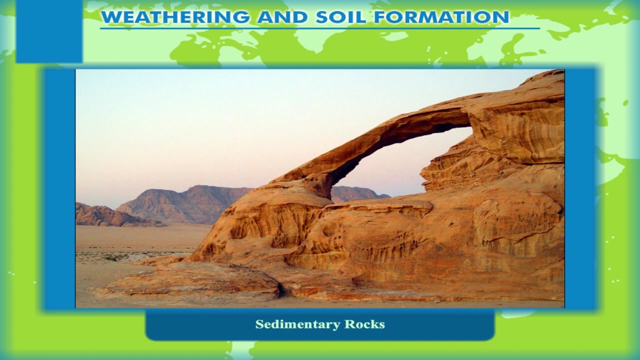 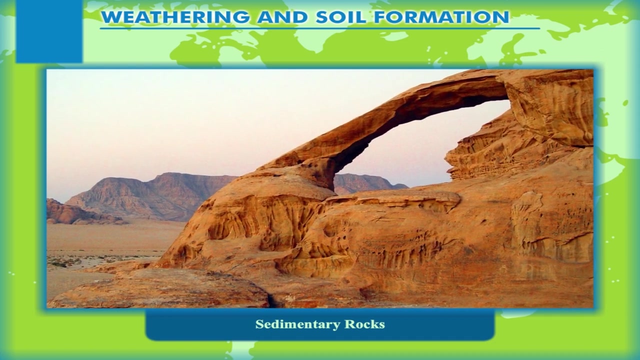 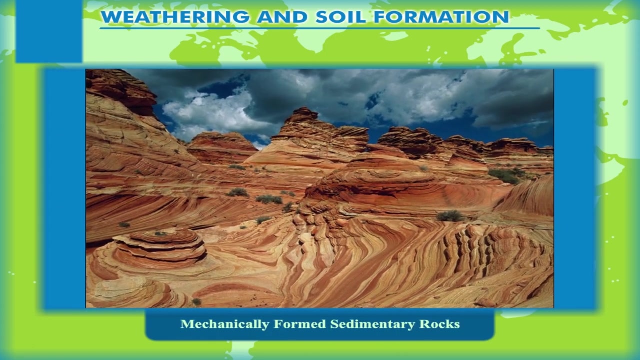 They are comparatively soft. These are formed when remains of vegetation and animals were buried and trapped within layers. They can be found in dry Claire's server. That is why or sedimentation can be classified as sedimentary rocks under three subtypes. fond of this, 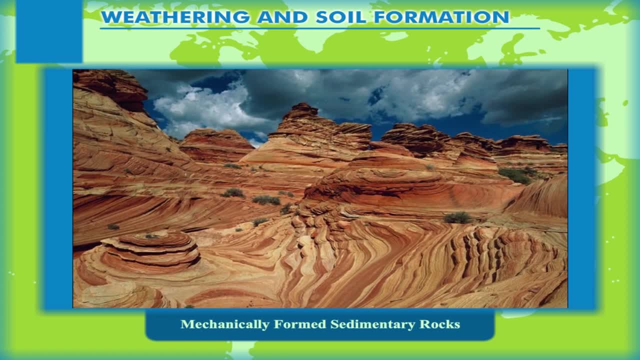 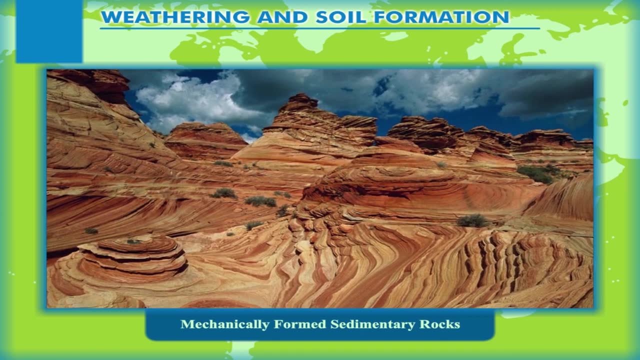 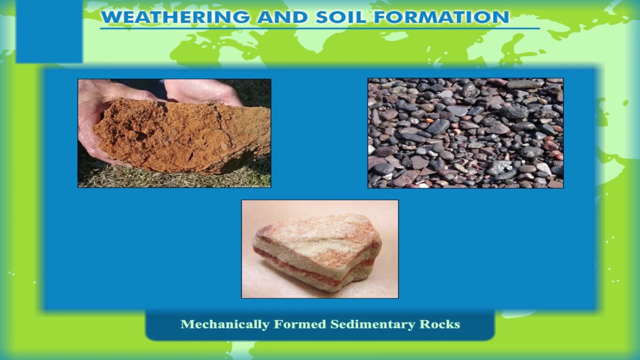 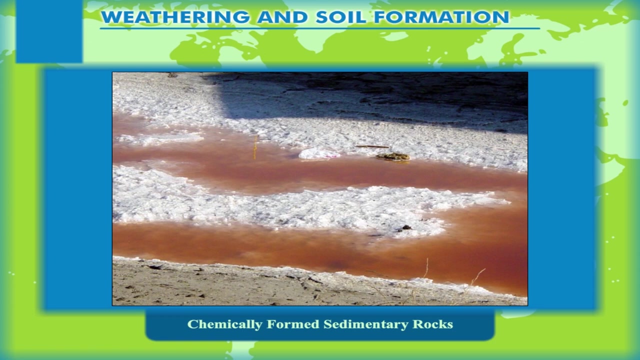 sedimentary rocks. When rocks are exposed to weather changes, they are broken and thus carried to a particular site, where such material is deposited in layers and the rocks are formed. Examples of such rocks are clay, gravel and sandstone. Chemically formed sedimentary rocks: They are formed by the process of evaporation of 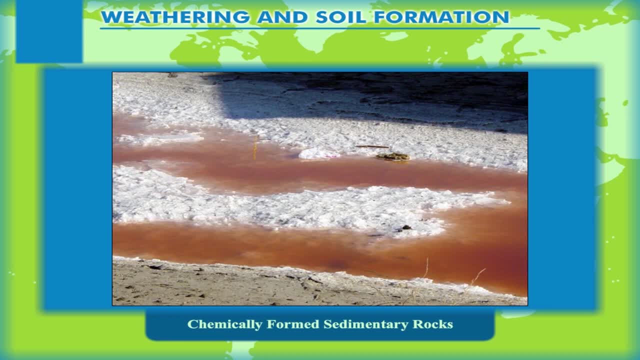 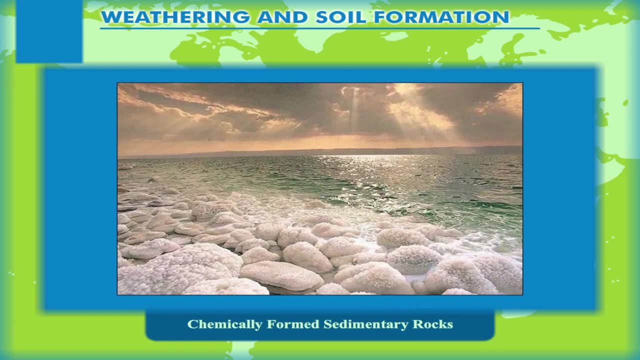 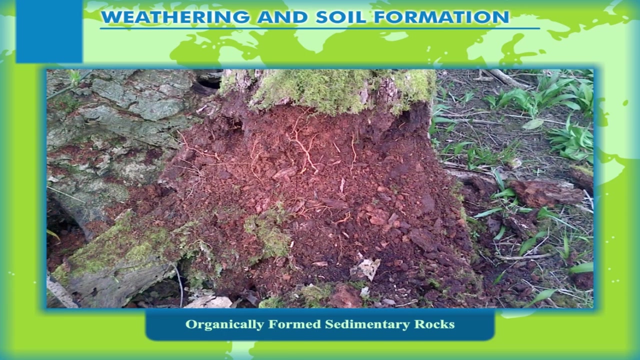 water containing mineral salt in solution. In deserts or shallow lakes, water evaporates, leaving behind a layer of salts. These salts get consolidated into sedimentary rocks. Examples of such rocks are common salt, gypsum and potash. Organically formed sedimentary rocks: They are formed by the accumulation of 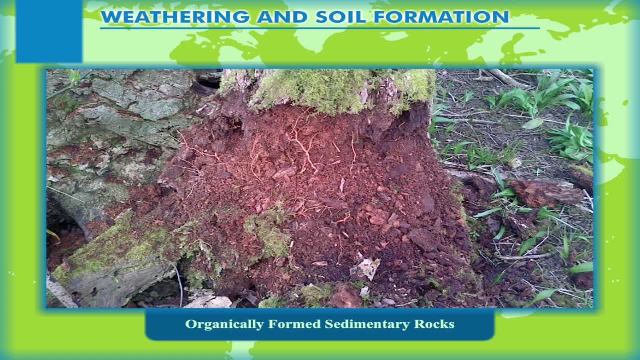 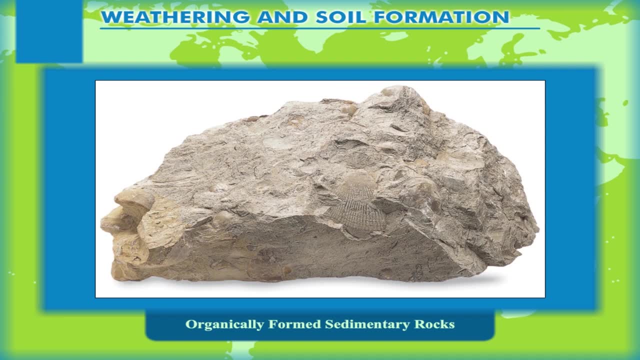 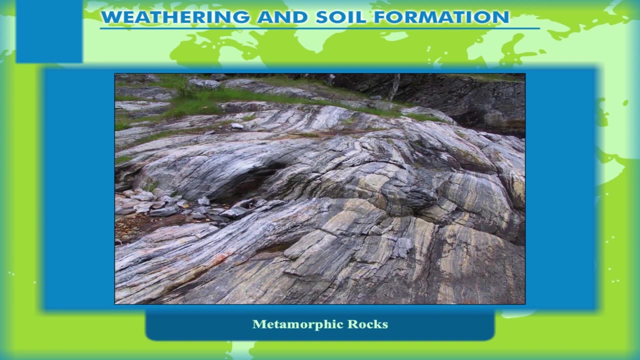 the remnant parts of organisms, plants and animals. Examples of such rocks are chalk, coal and limestone. Metamorphic rocks: The meaning of metamorphic is changed or altered. These rocks are either igneous or sedimentary rocks which have undergone a change due to excessive heat or pressure. 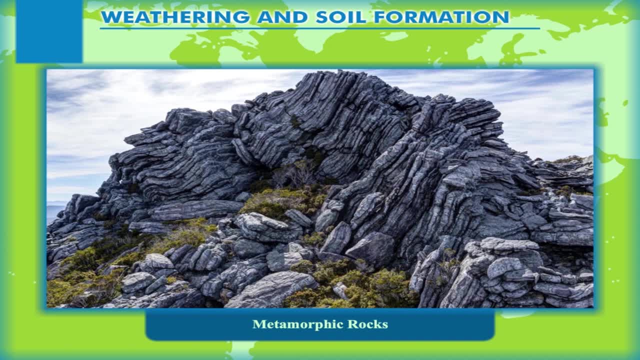 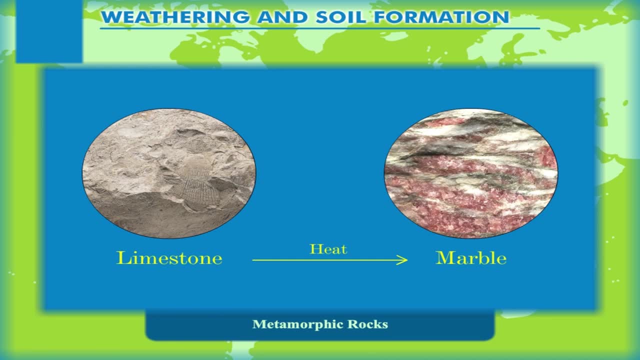 This change of one type of rock is called a metamorphic rock. One type of rock to another is called metamorphic rocks. For example, due to excessive heat, limestone, changes into marble and sandstone, changes to quartzite, Metamorphic rocks are: 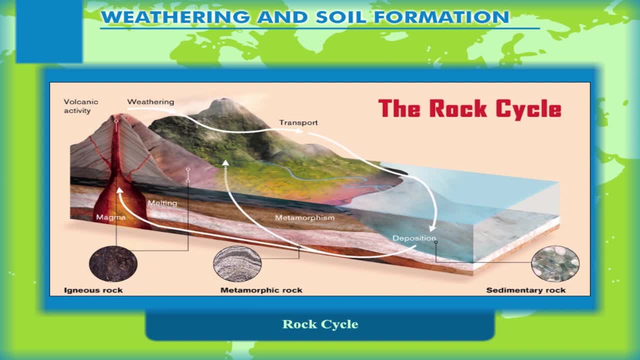 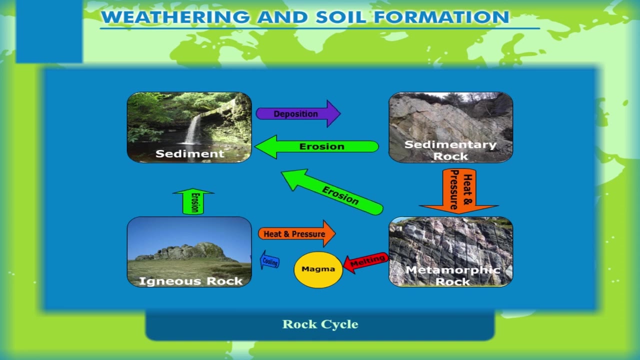 very hard Rock cycle. The three categories of rocks are constantly forming from one another in a continuous circuit, which is known as rock cycle. When igneous rocks are exposed to weather changes, they are broken and eroded and give birth to sedimentary rocks Due to excessive pressure. 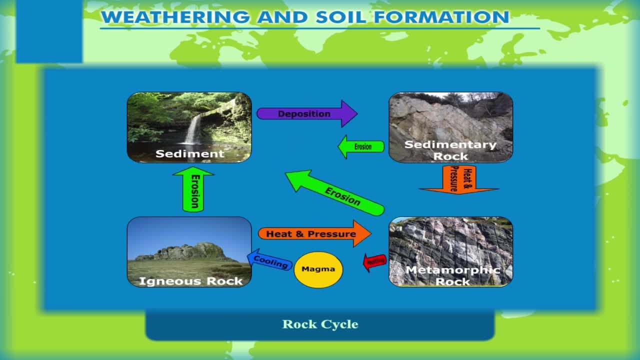 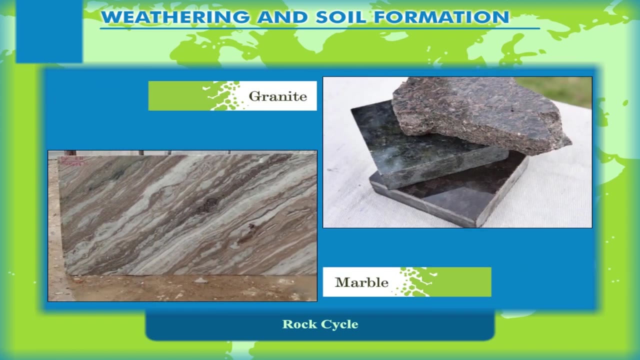 and heat, these rocks further undergo a change into metamorphic rocks. Thus, this cycle of change from one type of rock into another is called rock cycle. Rocks can be used for various purposes: As building materials, marble and granite- or fuels, coal, iron or metal. These are the portions of rock that become metamorphic rocks.